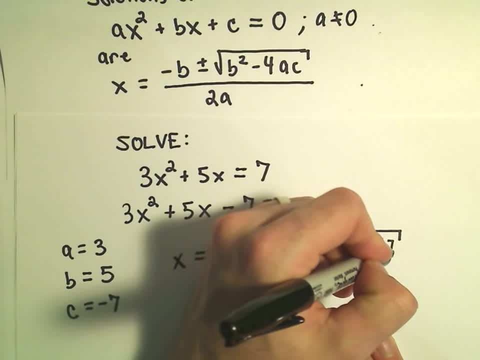 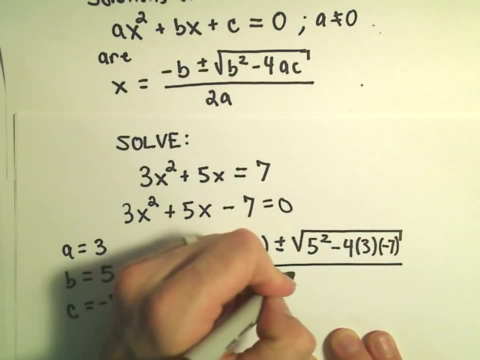 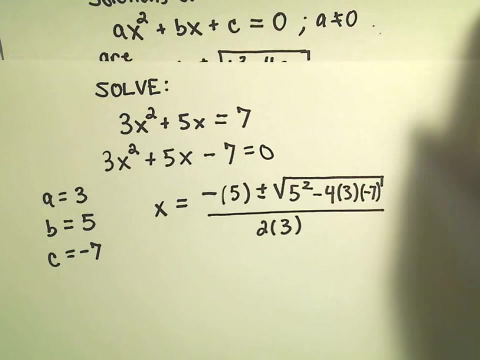 times our c value, which we said was negative 7, and then that's all going to be divided by 2 times a, or in this case, 2 times 3.. So now it's just a matter again of simplifying down this expression and, you know, just trying to reduce it if you can. 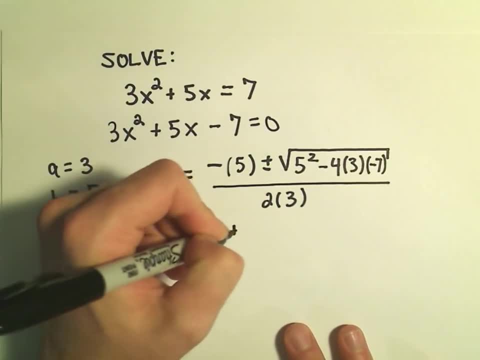 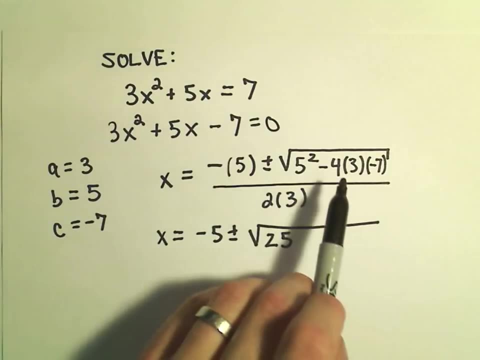 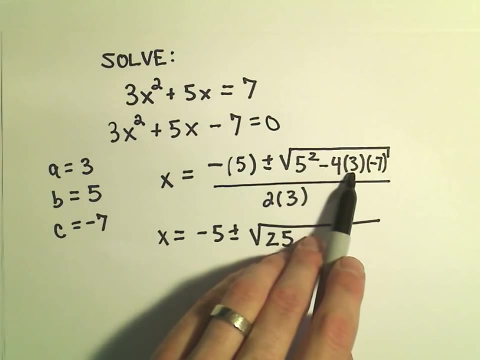 So we have x equals, we'll have negative 5, plus or minus the square root. let's see. so 5 times 5 is 25, and then we have negative 4 times 3 times negative, 7, so negative 4 times positive, 3 is going to be negative 12,. 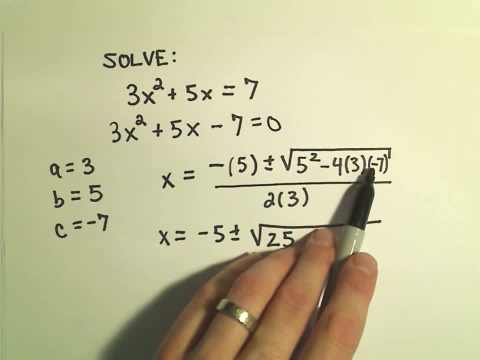 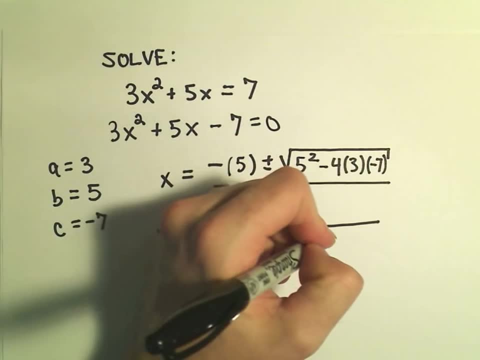 negative 12 times positive- excuse me, times negative 7, so we have negative 12 times negative. 7 will give us a positive, and then 12 times 7 is going to give us 84, and that's all divided by 2 times a or 6,. 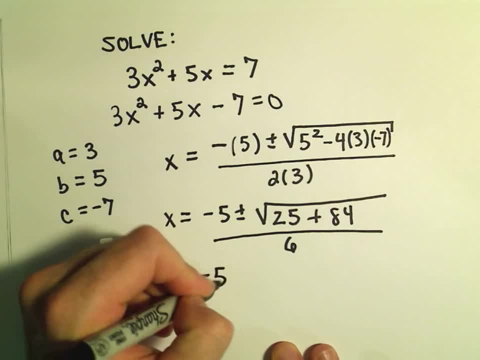 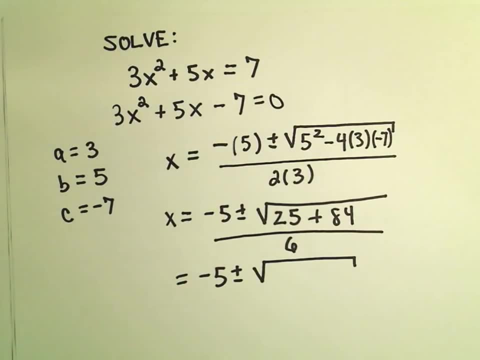 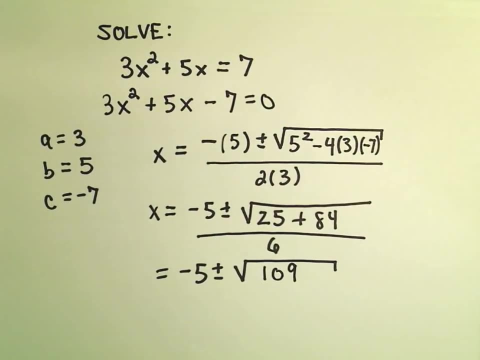 so we have negative 5 plus or minus the square root, so let's see 25 and 84, so I believe that's going to give us positive 109 when we add those together, and all of that's going to be divided again by 6,. 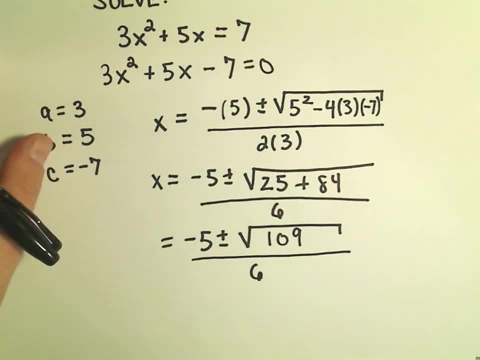 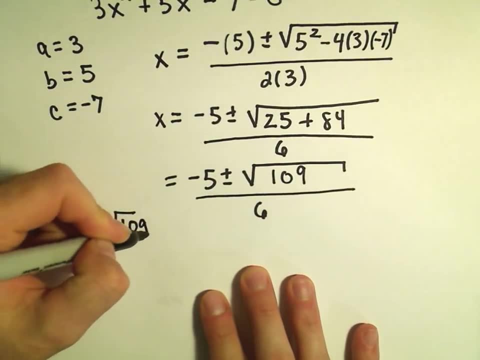 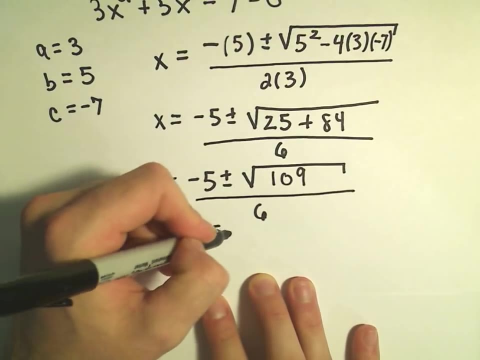 and if you wanted to again, we can kind of break this down into our two separate statements. so we've got negative 5 plus the square root of 109 divided by 6 as one solution. our other solution will be negative 5 minus the square root of 109 divided by 6,. 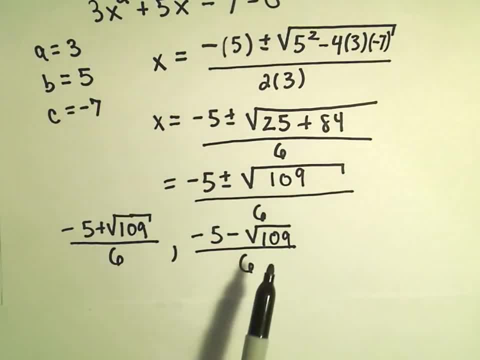 and here we can start trying to break down 109, trying to reduce it a little bit. but I think if you play with it a little bit, you know maybe you'll find something that divides into it. but to me I'm pretty sure that 109 is actually a prime number. 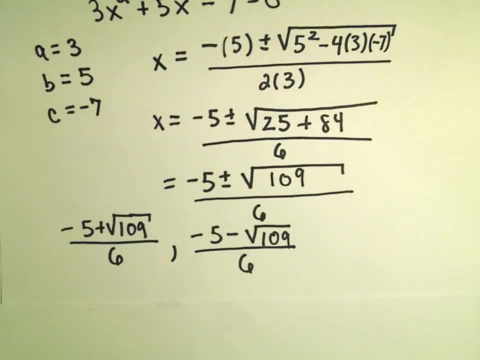 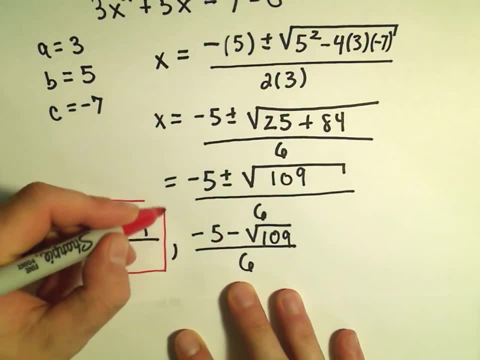 so this isn't going to factor any further. we're not going to be able to reduce it in any kind of meaningful way, so to me, these would simply be our two solutions: negative 5 plus the square root of 109 over 6,. 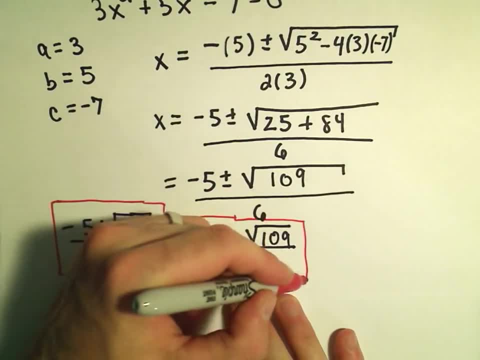 and negative 5 minus the square root of 109 over 6..